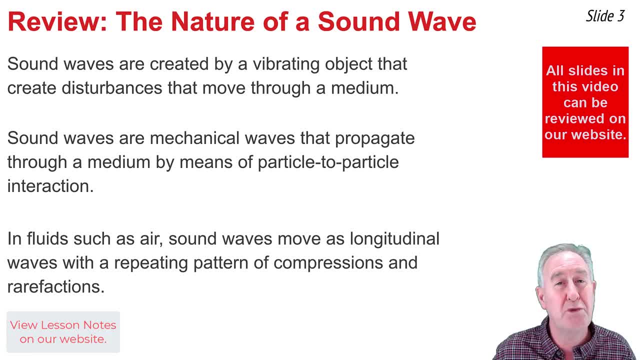 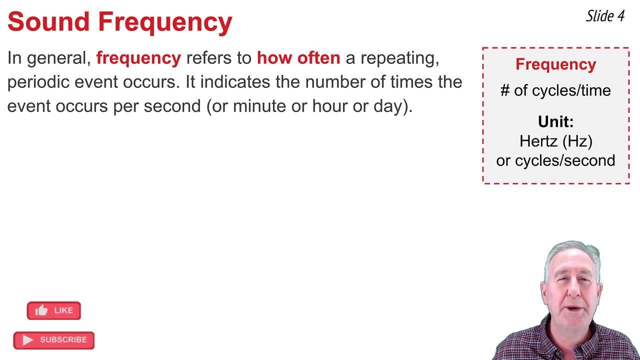 compressions and rarefactions is what we observe moving through the medium. Finally, a sound wave transports energy from one location to another without actually moving physical matter. Frequency is one property of a sound wave. In general, the word frequency refers to how often. 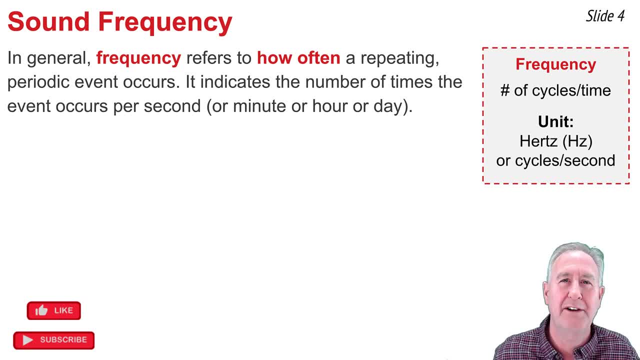 a periodic and repeating event repeats itself. It indicates the number of times the event occurs: per second, per minute, per day, per year. If the event happens to be the orbit of the earth about the sun, we would describe its frequency as one time per year. For waves, the event happens. 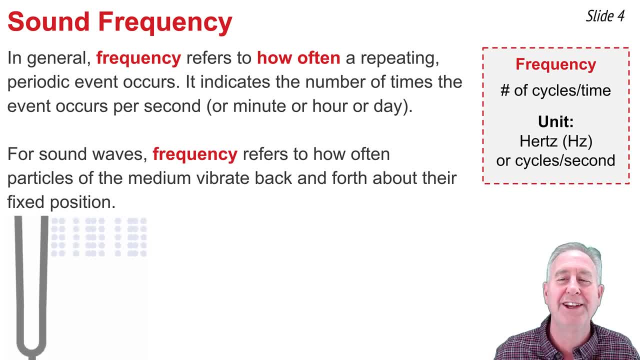 to be a vibration of a particle about its fixed position. So for sound waves, frequency refers to how often a particle repeats one complete back-and-forth vibrational cycle. We measure it in cycles per time, such as cycles per second. An equivalent unit would be the unit Hertz. 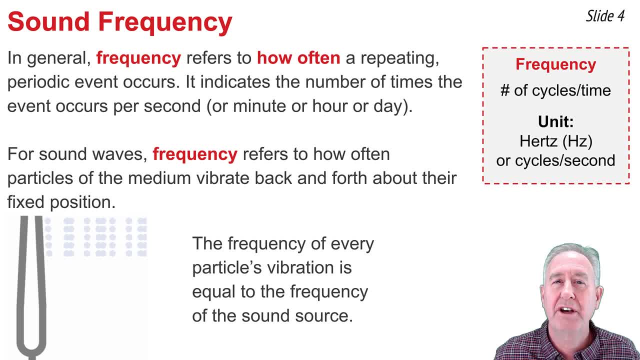 abbreviated HZ. One thing you can be certain of is that the vibrational frequencies of the particles of the medium are perfectly synchronized with the vibrational frequencies of its source. So if the source of a sound wave is a tuning fork vibrating back and forth, 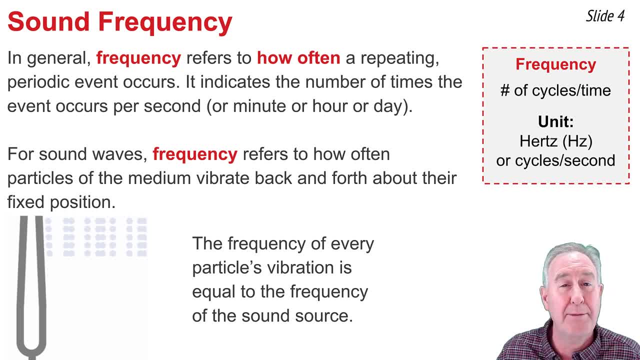 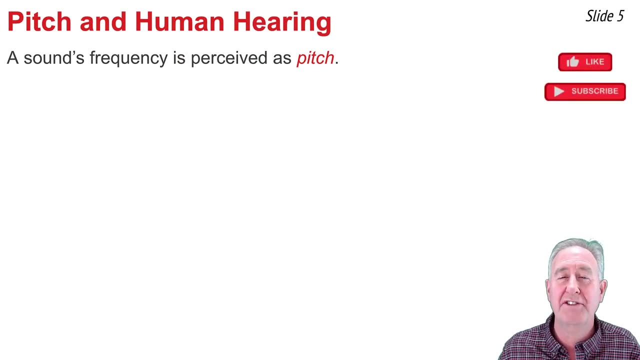 then you can be certain that if the tines of the tuning fork vibrate back and forth 260 times per second, then every particle of the medium will vibrate back and forth 260 times per second. A sound's frequency is perceived as its pitch, a quality of sound that 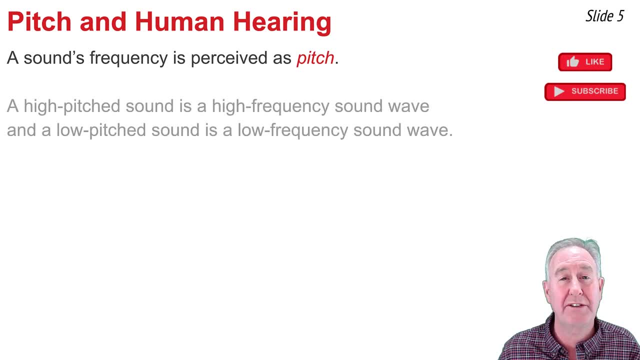 many of us don't know about. So if a sound wave is a tuning fork vibrating back and forth, a high-pitched sound is perceived of a high-frequency sound wave and a low-pitched sound is perceived of a low-frequency sound wave. Humans can typically hear frequencies that are as 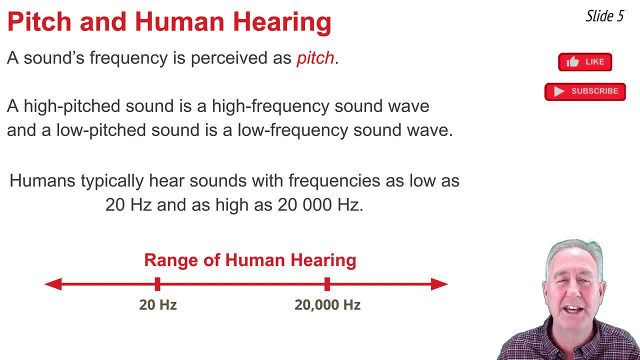 low as 20 Hertz and as high as 20,000 Hertz. This is referred to as the audible range of human hearing. A sound with a frequency less than 20 Hertz is an infrasonic sound and a sound with a frequency greater than 20,000 Hertz is an ultrasonic sound. So if a sound with a frequency 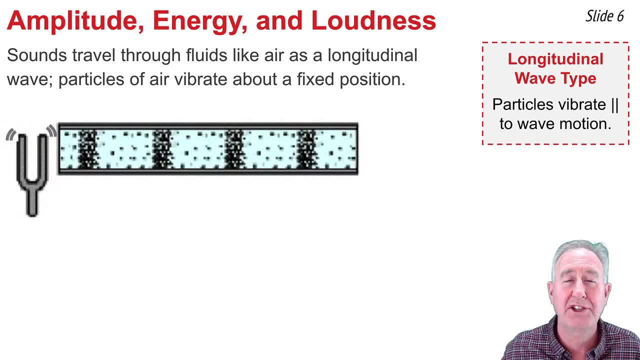 less than 20 Hertz is an infrasonic sound, then a sound with a frequency less than 20 Hertz is an ultrasonic sound. Sound travels through fluids such as air as a longitudinal wave. The particles of the medium vibrate back and forth in a direction that is parallel and anti-parallel. 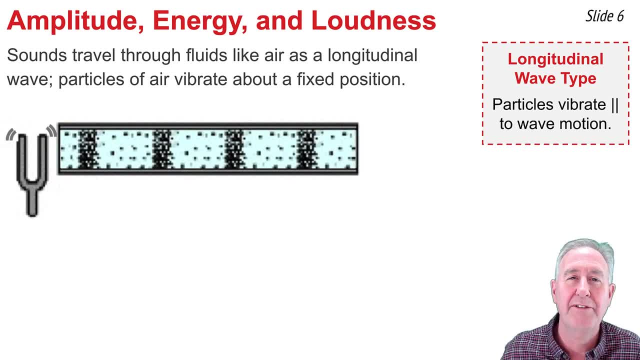 to the direction that the wave is traveling. So if a wave is traveling from a tuning fork as its source, from left to right, particles of the medium vibrate back and forth, left to right and right to left. This creates compressions and rarefactions within the medium. This pattern of compressions and 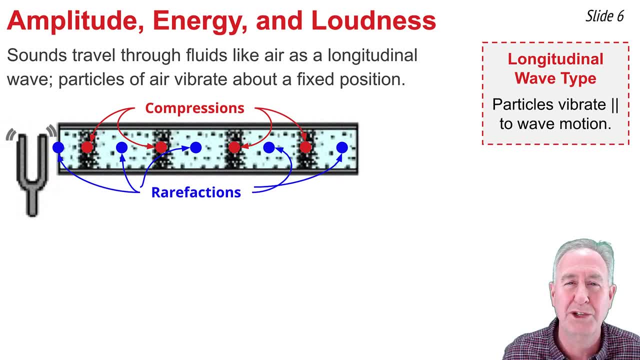 rarefactions is what we observe moving from the source to the surrounding regions. The amplitude refers to the maximum displacement of a particle from its rest position. So if I were to isolate a single particle and watch it vibrate from rest to a far right position and then back to a far left, 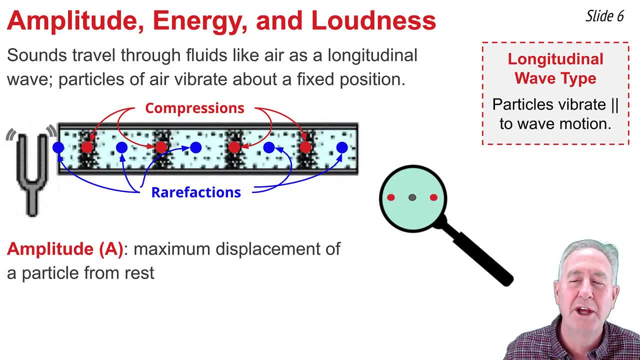 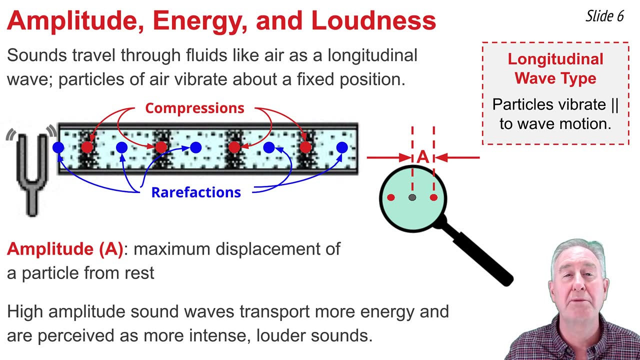 position and back to a far right position, and so forth. we would describe the amplitude as being the distance from the rest position to the far right position, Or from the rest position to the far left position. Now, if I were to whisper the particles of the, 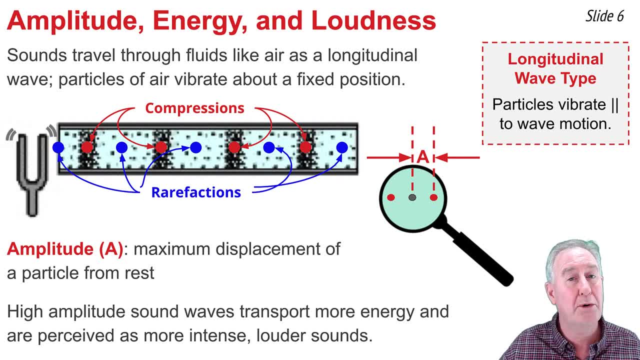 medium would vibrate with a small amplitude, I'd be putting very little energy into the wave. There'd be very small amplitude and you would perceive it as a soft, not loud, sound. But if I were to holler, I would be putting a lot of energy into the wave. We would observe the amplitude to be significantly. 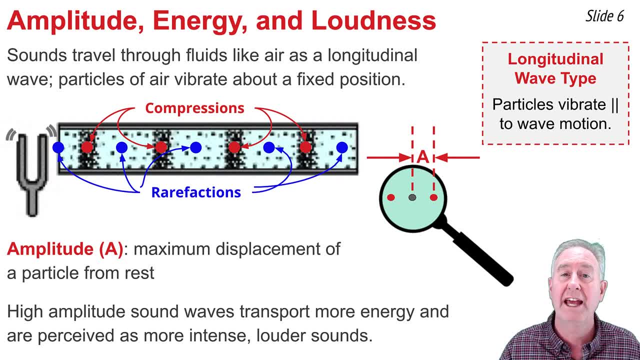 greater and that sound would be perceived as a soft, not loud sound. So if I were to holler, it would be perceived as a loud or intense sound. So high amplitude sounds are associated with sounds that transport a lot of energy and are perceived as loud, intense sounds. 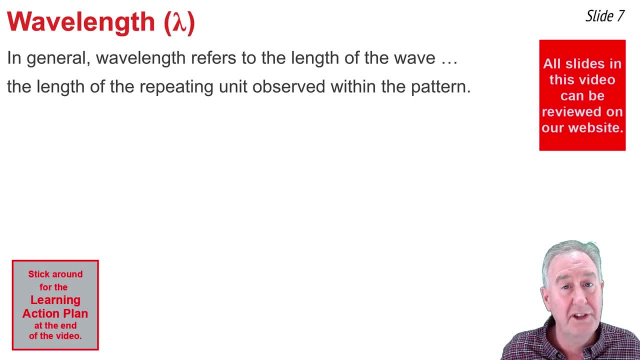 In general, wavelength is the length of a wave. It's the length of the repeating unit that's observed within the wave pattern. We typically think of it as the distance from crest to crest or the distance from trough to trough, But longitudinal waves, like a sound wave moving. 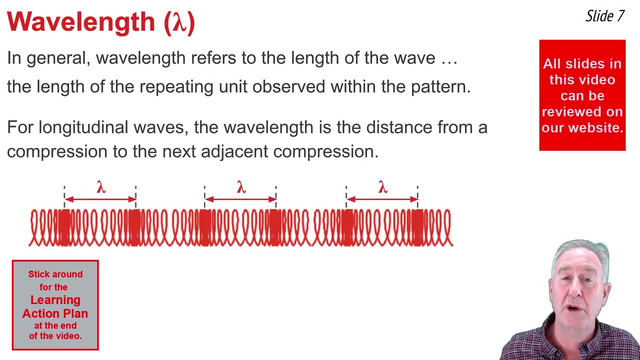 through air don't have a long wavelength, So we would think of it as the length of the. don't have crests and troughs. Instead they have compressions and rarefactions. Here we see a diagram of a longitudinal wave moving through a slinky, and the wavelength could be thought of. 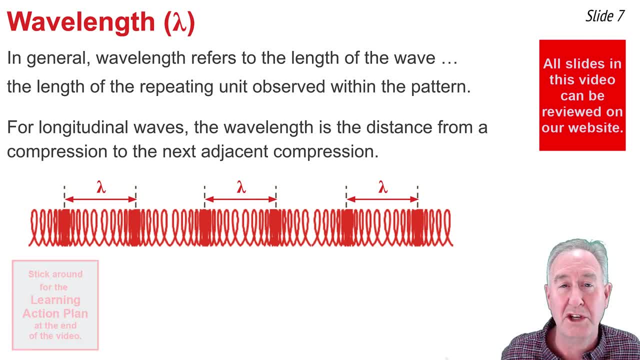 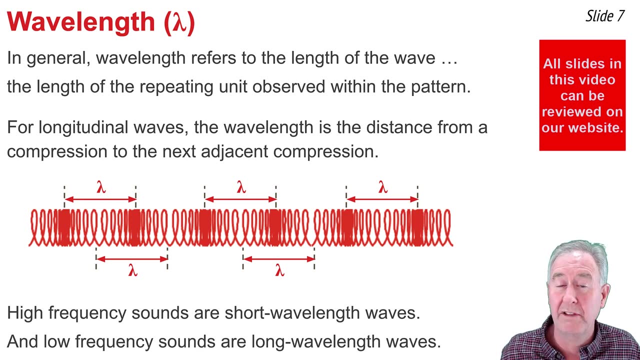 as the distance from one compression to the next adjacent compression or, just as equally, the distance from a rarefaction to the next adjacent rarefaction. Wavelength and frequency are inversely related to one another. A high-frequency sound wave is a short wavelength wave and a low-frequency. 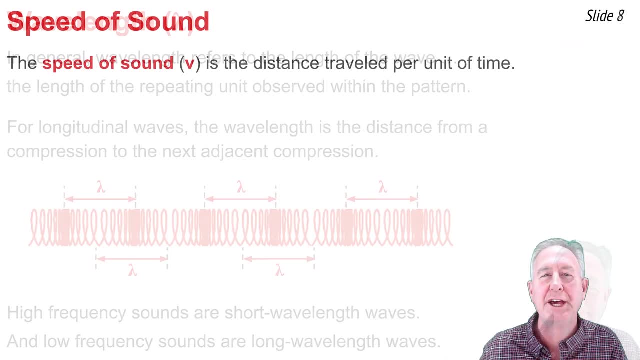 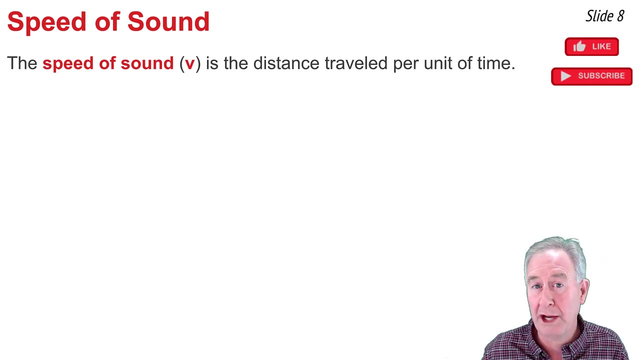 sound wave is a long wavelength wave. The speed of sound, like the speed of any object, is the distance traveled per unit of time. It's the distance a compression of the sound wave would travel in some amount of time. The speed of sound is dependent upon the properties of the medium. 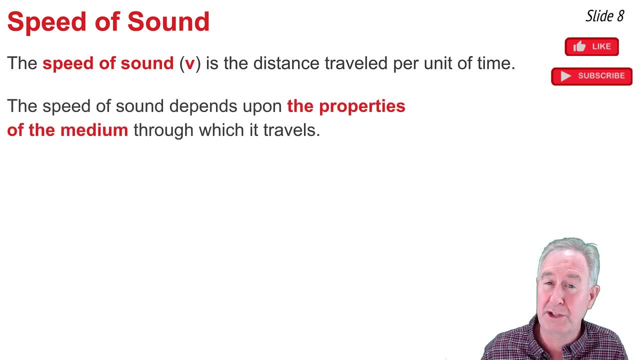 One property would be the state of matter: solids, liquids versus gases. We could assert that in general, that the speed of sound within a solid is greater than that within a liquid and is greater than that within a gas, For instance, the speed of sound traveling. 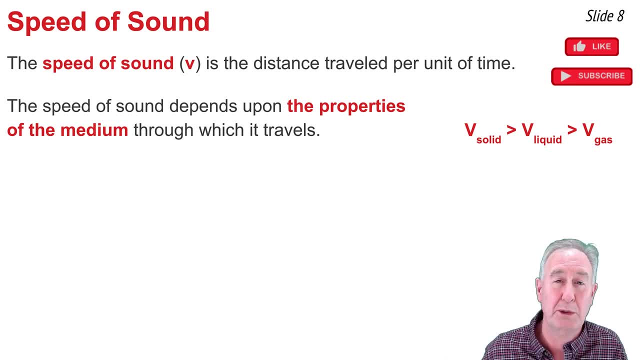 through the solid aluminum is about 5,100 meters per second, but the speed of sound traveling through the liquid water is about 1,400 or 1,500 meters per second, And for sound traveling through the gas air it's about 340 or 350 meters per second. 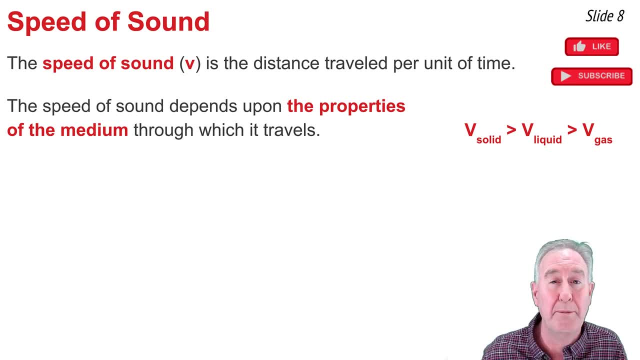 When it comes to a sound wave traveling through air, the main property that affects its speed would be the temperature, And we could write an equation that expresses the speed of sound in air as a function of temperature. It would look something like this: The speed of sound is: 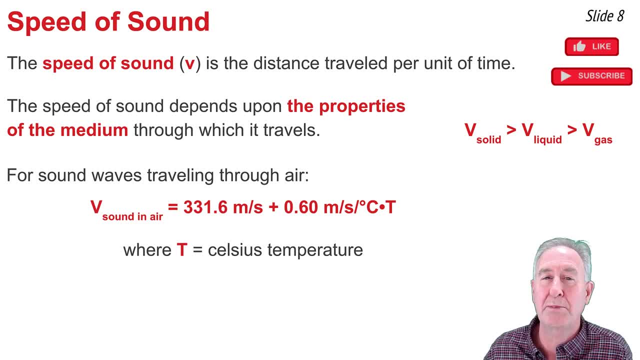 331.6 meters per second, plus 0.6 times the temperature in degrees C. If we were to substitute 20 degrees into this equation, we would get about 343.6.. The speed of sound is not dependent upon the frequency, wavelength or amplitude of the sound. 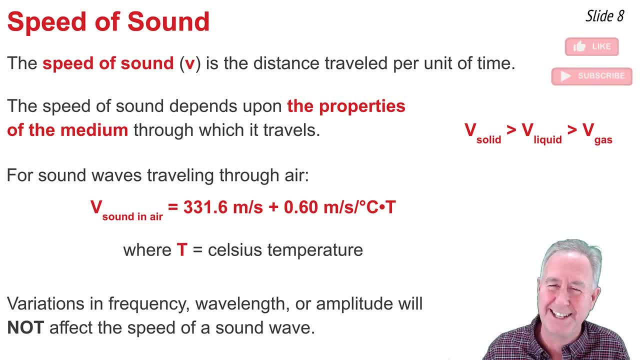 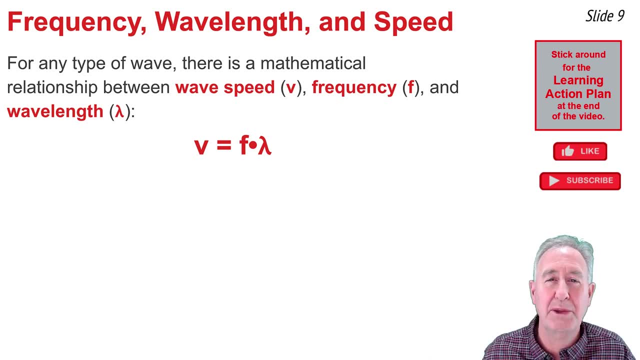 wave and fully dependent upon the properties of the medium. For any type of wave, there is a mathematical relationship between the wave speed, the frequency and the wavelength, as given by this equation: v equal f times lambda. The speed of a wave is dependent upon the properties of the 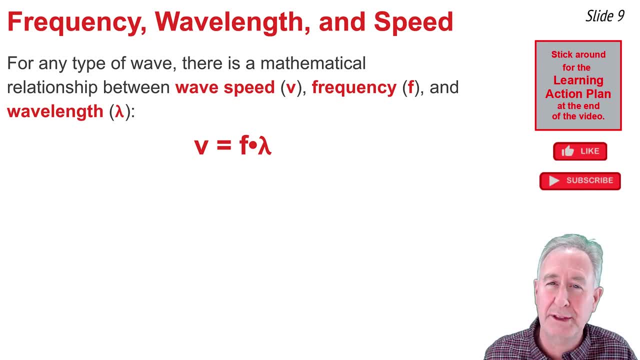 medium and unaffected by variations in the frequency, wavelength and temperature. So for a wave traveling through a uniform medium, we could say that the left side of this equation is a constant value and a variation of the frequency would not affect the speed, but instead